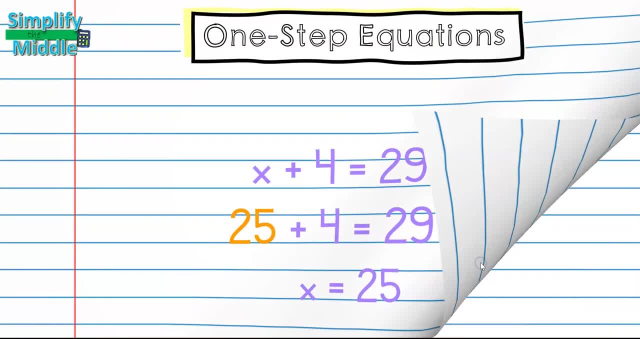 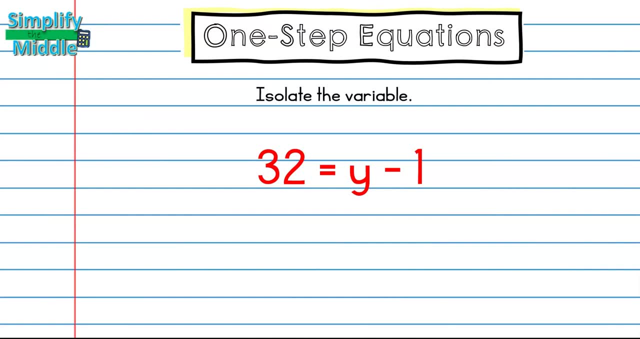 plus 4 needs to equal 29,. and it does My next problem: 32 equals y minus 1.. I will still always be isolating my variable, and I'm going to do that by asking what operation is being done to the variable. Well, this time the variable is on this side and the operation being done to 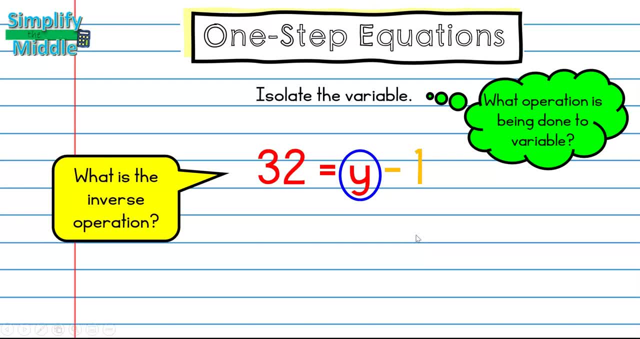 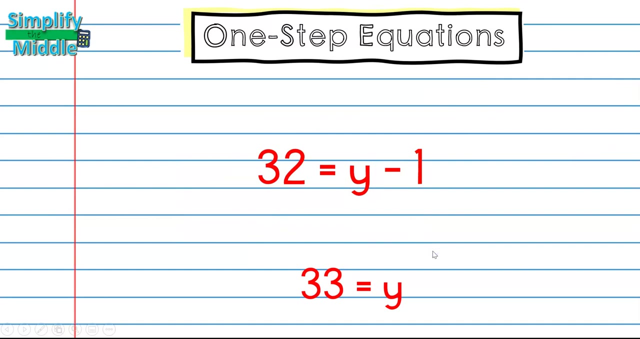 it is subtracting by 1.. So what is the inverse of subtraction Addition? So I'll add 1 to both sides this time. This time this side is going to cross out because I have negative 1 plus 1, which is 0. So my answer is 32 plus 1, which is 33 equals y. Remember I can substitute that in. 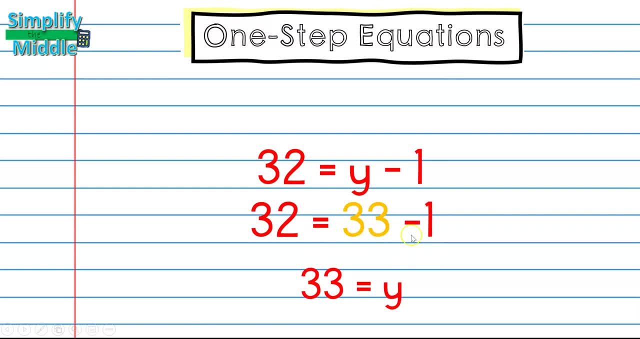 for y and see if I'm correct, 32 equals 33 minus 1,, which is 32 plus 1,, which is 33 minus 1,, which is 33 plus 1, and it does. For this problem, I will still isolate the variable, which, in this case, is: 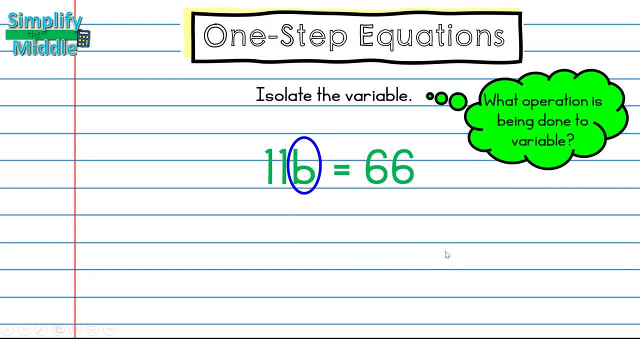 on this side It's b. I'm going to ask what operation is being done to the variable. Well, I see there's an 11 outside here of a coefficient of 11. Remember, when a variable is next to a number, and that means it's a coefficient, it means to multiply. So what is the inverse of? 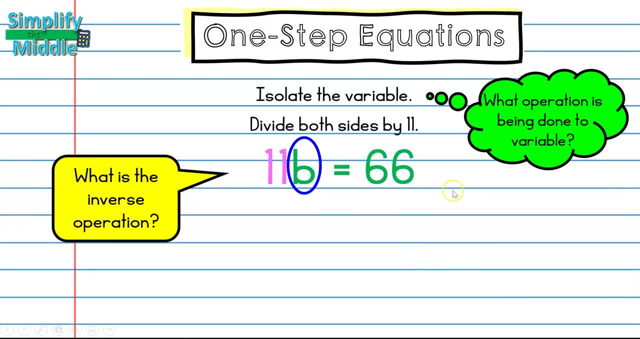 multiplication Addition. So what is the inverse of multiplication Addition? So what is the inverse multiplication Division? So I'm going to divide both sides by 11.. I always want to use a fraction bar to show division with equations instead of using the normal division symbol, So I'm just 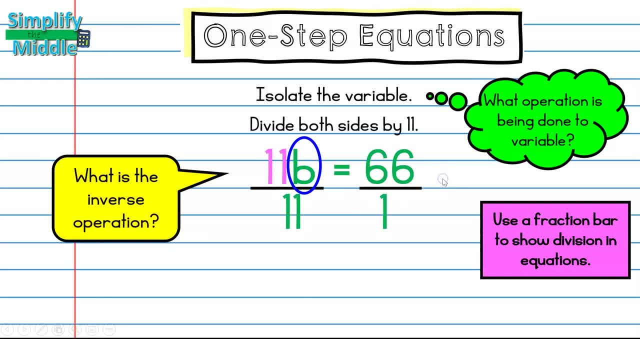 going to draw a fraction bar under each of these terms and I'm going to write 11 underneath to show that they're being divided by 11.. So I will have b equals 6.. The reason that these are going to cancel out is because 11 divided by 11 is 1.. 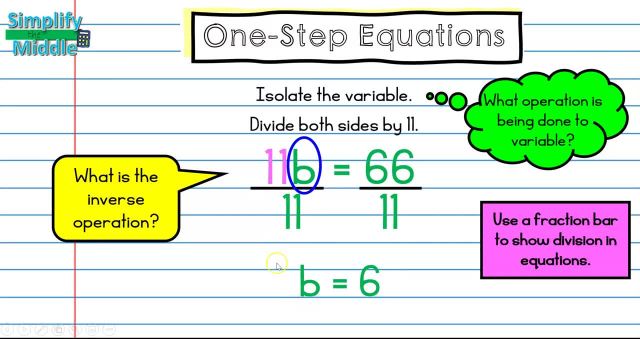 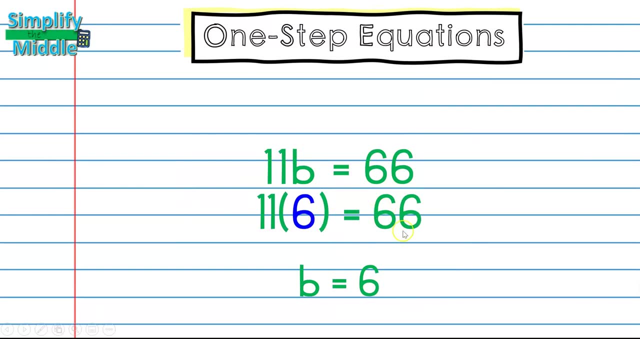 And we know that there is a coefficient of 1 in front of all variables that have no number in front of them normally. So this makes sense: 1b is equal to 6, or just b is equal to 6.. Remember, I can substitute that answer in, and 11 times 6 is 66. So I'm correct.